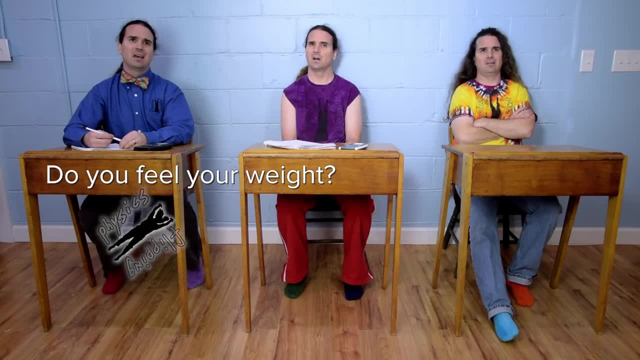 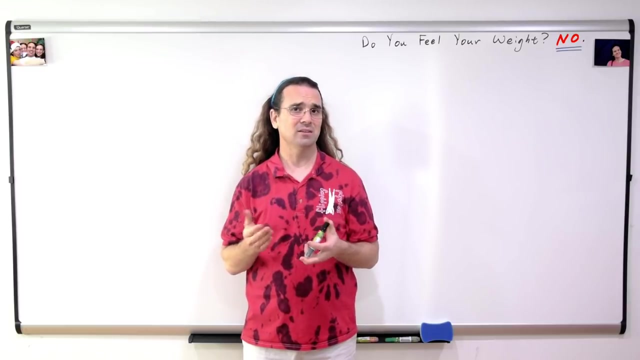 Mr, Good morning. Do you feel your weight? Flipping Physics, Mr. Of course I feel my weight. Are you daft or something? Uh, no, Actually you do not feel the force of gravity acting on you. You do not feel your weight. 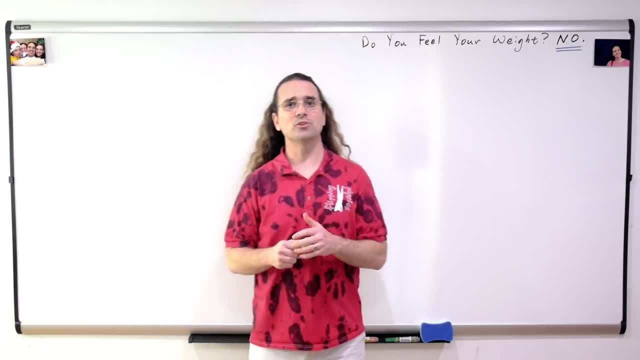 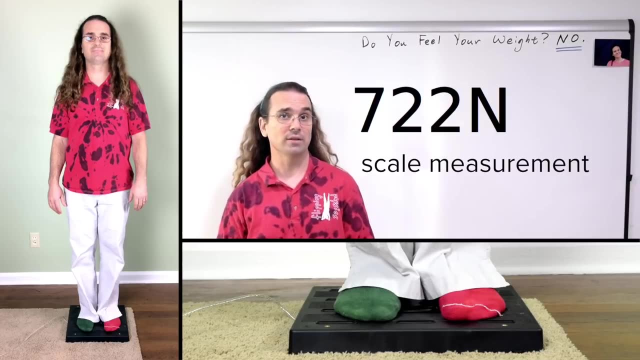 That makes no sense, Wrong, Mr? Okay, I will prove it to you. When you stand on a scale, people often think the scale is measuring the force of gravity acting on you, or what we call your weight, When you are standing on the surface of the Earth. 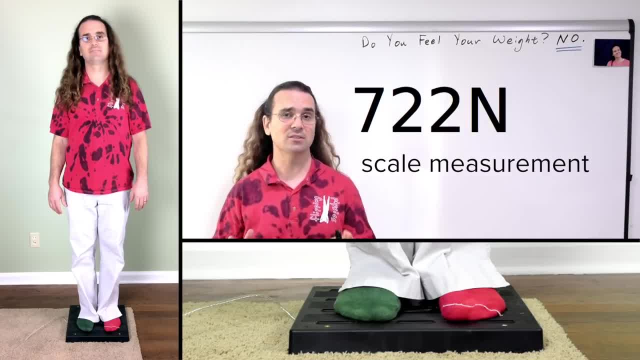 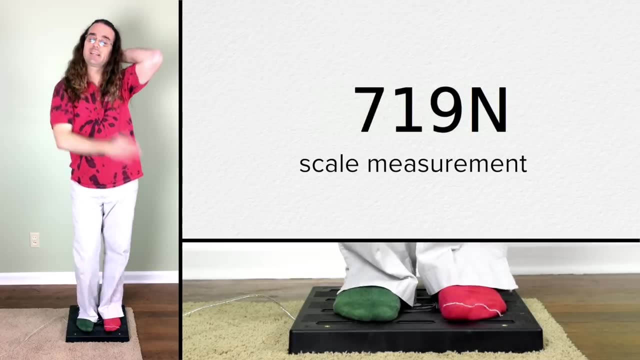 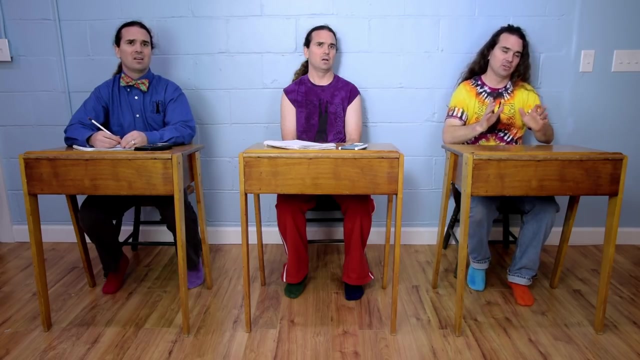 the force of gravity caused on you by the Earth is constant. It does not change. If the scale measures my weight, why does the reading on the scale change when I dance? Hey, Macarena, aye, Mr. Okay, I get it. 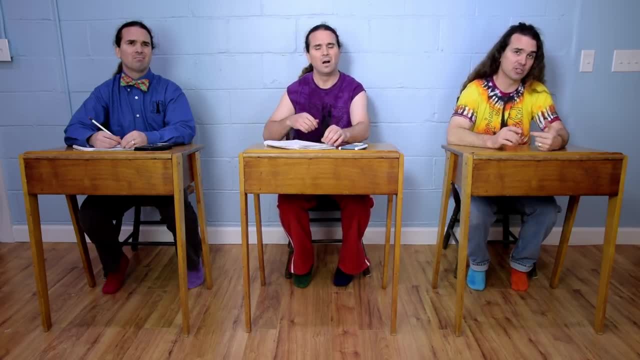 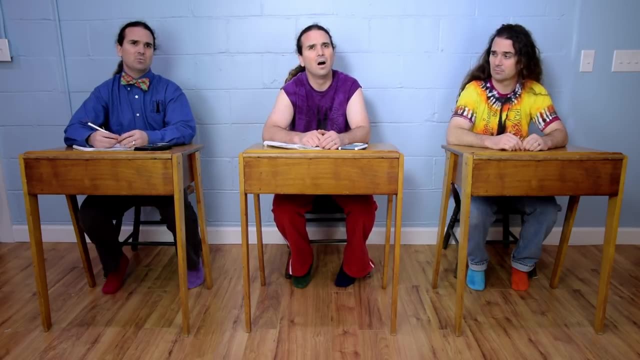 Your weight is constant, even when you dance. However, the measurement on the scale changes as you dance, so the scale does not measure your weight. But if the scale does not measure your weight, what does it measure? Mr Good question. The scale measures the downward force you apply to it. 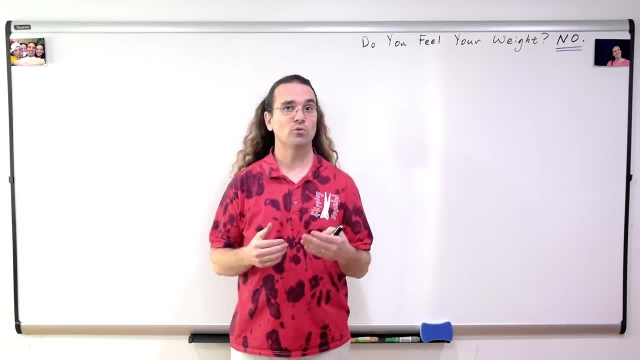 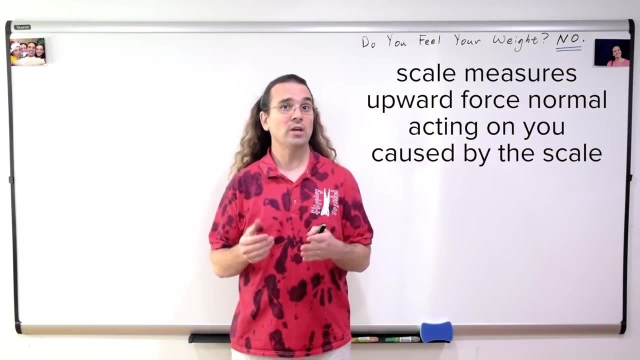 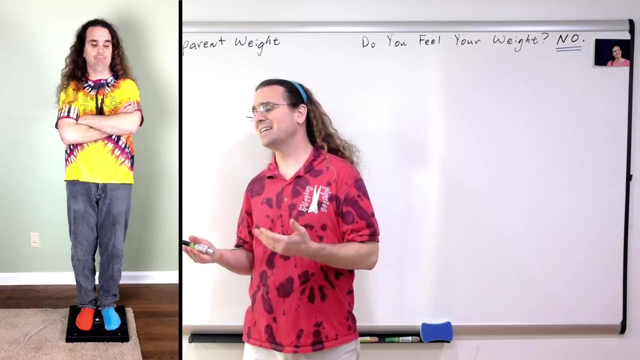 which, according to Newton's Third Law, is equal and opposite to the force normal acting on you. In effect, the scale measures the force normal acting on you, which we also call your apparent weight. Okay, Bo, let's analyze you standing on a scale. 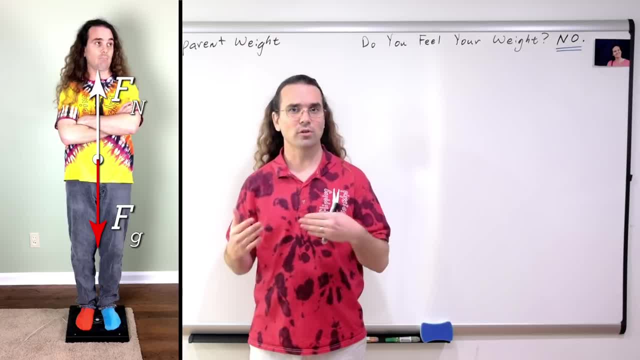 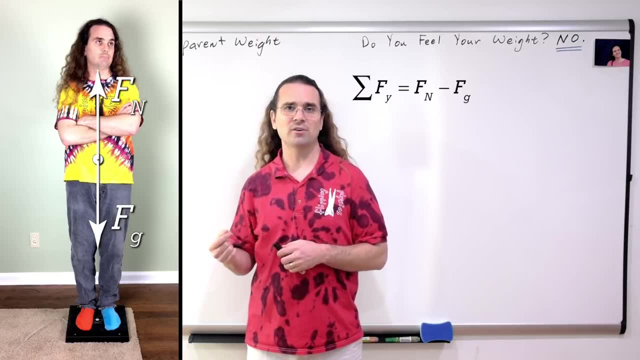 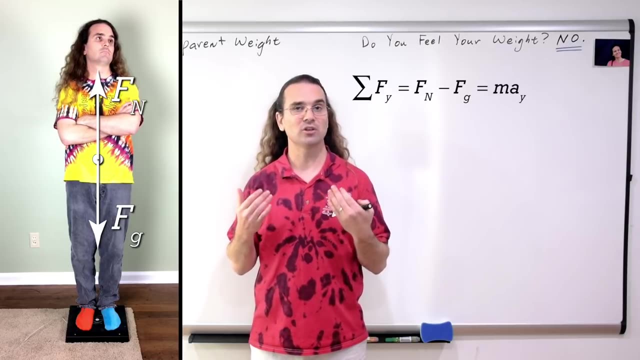 The forces acting on you are your weight or the force of gravity which is down, and the force normal which is up. Newton's Second Law says the net force in the y-direction equals force normal minus force of gravity, and the net force in the y-direction also equals mass times. acceleration in the y-direction. 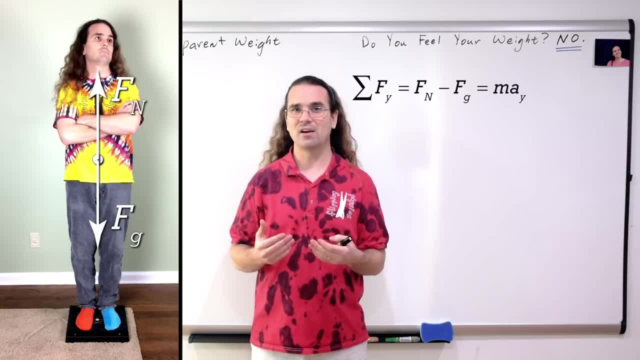 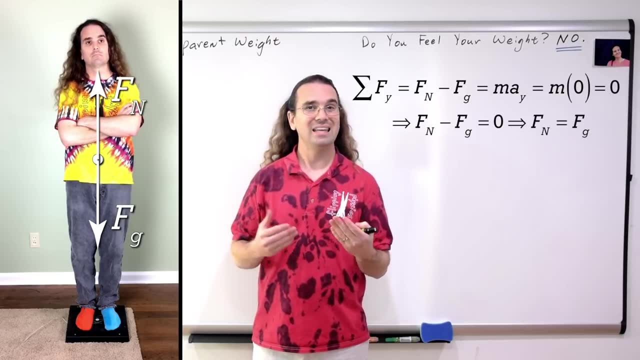 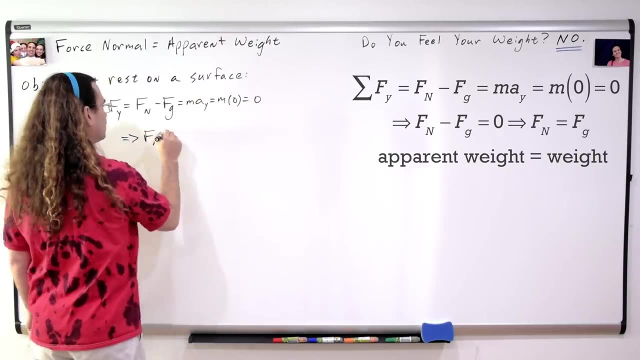 In a typical situation where you are just standing there at rest, your acceleration in the y-direction is equal to the acceleration in the y-direction. Your acceleration in the y-direction is zero. so your force normal equals your weight Bo. in that situation, your apparent weight and your weight are the same. 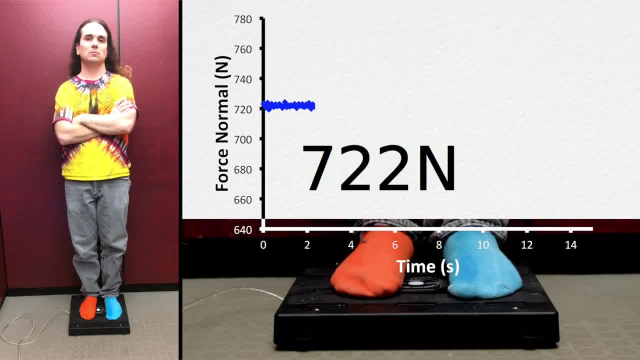 Bo, now let's put you in an elevator which is about to move upward. Okay, it just started to move upward and now is moving at a constant velocity, And now it has stopped. Bo, please describe what your weight felt like while that was happening. 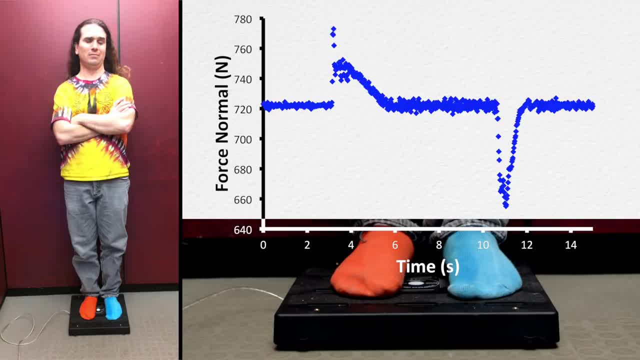 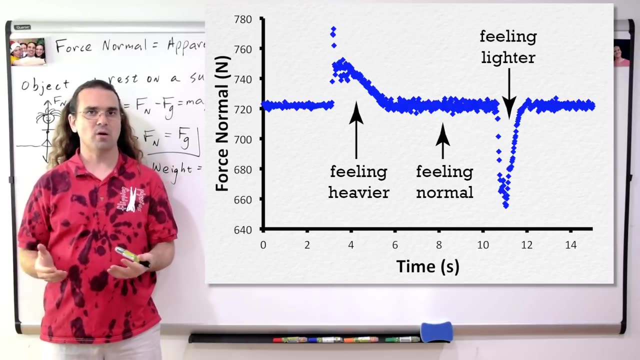 Okay, how did my weight feel For a brief moment? when the elevator started up? I felt heavier than normal. Then I felt normal for a bit, And then, when the elevator stopped, I felt lighter for just a second. Okay, at the beginning, let's call it part one. 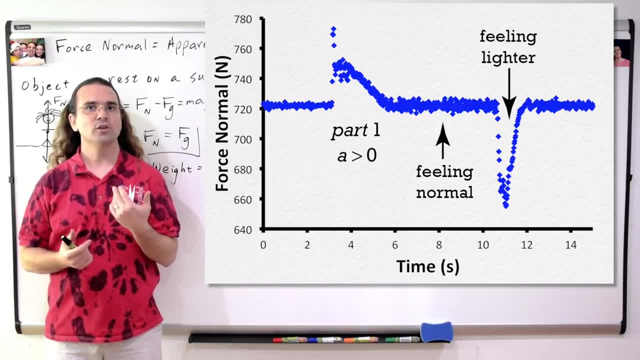 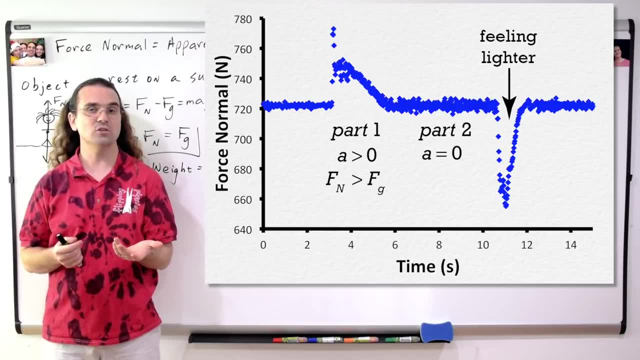 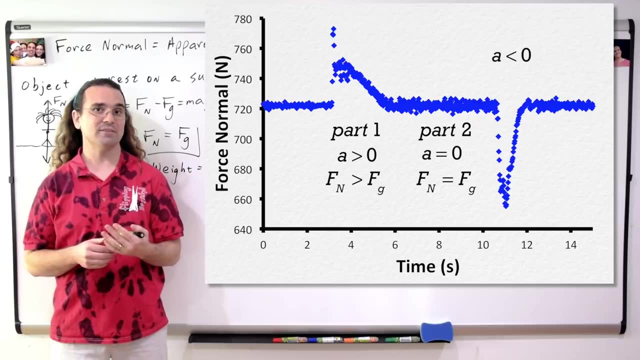 when you had an upward or positive acceleration, your apparent weight was more than your weight. And then, as the elevator and you were moving at a constant velocity- let's call it part two- your apparent weight was the same as your weight. And at the end, when you had a downward or negative acceleration, let's call it part three. 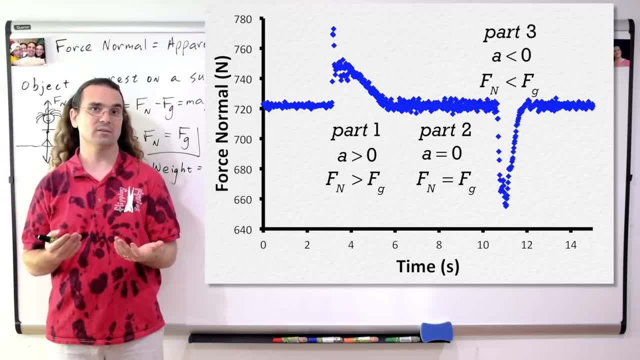 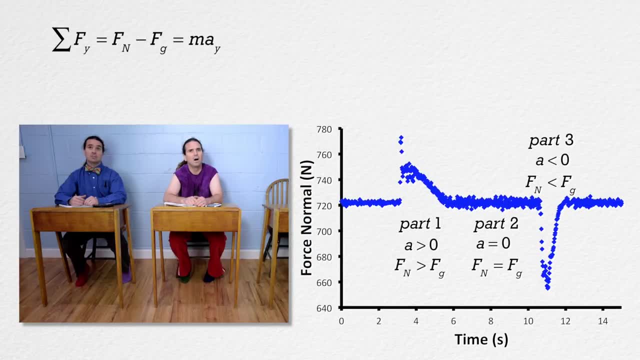 your apparent weight was less than your weight. Billy, could you please explain this? Okay, going back to the free body diagram and Newton's second law, Add force of gravity to both sides of the equation and we get force. normal equals force of gravity. 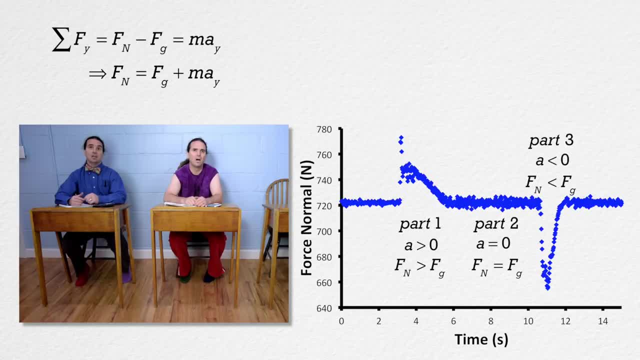 plus mass times acceleration in the y direction. In other words, in this specific situation, apparent weight equals weight plus mass times acceleration in the y direction. Okay, so during part one, Bo, when you are just starting to move upward, you have an upward or positive acceleration and therefore mass times acceleration in the y direction is a positive number. 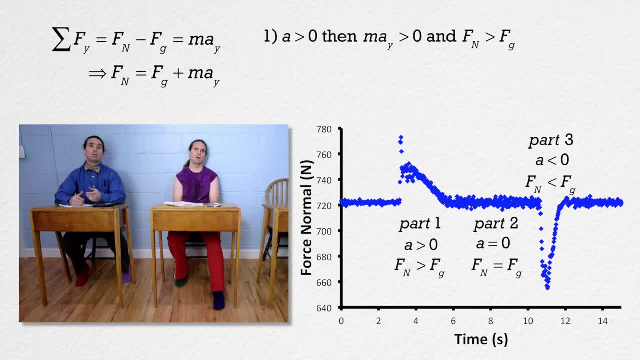 and your apparent weight is greater than your weight, Which is why you feel heavier as the elevator starts moving upward. During part two, when you are moving at a constant velocity, your acceleration in the y direction is zero and your apparent weight and your weight are equal. 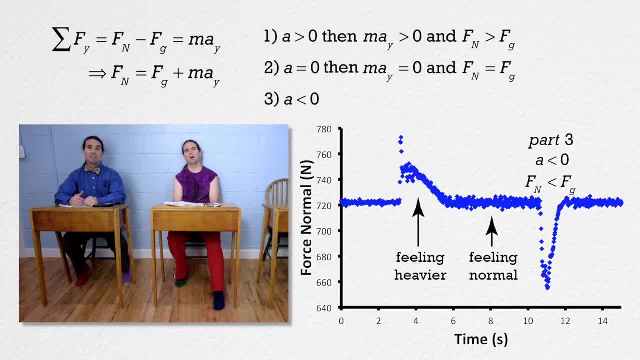 During part three, when the elevator is stopping, you have a downward or negative acceleration and therefore mass times. acceleration in the y direction is a negative number and your apparent weight is less than your weight, Which is why you feel lighter as the elevator stops moving upward.